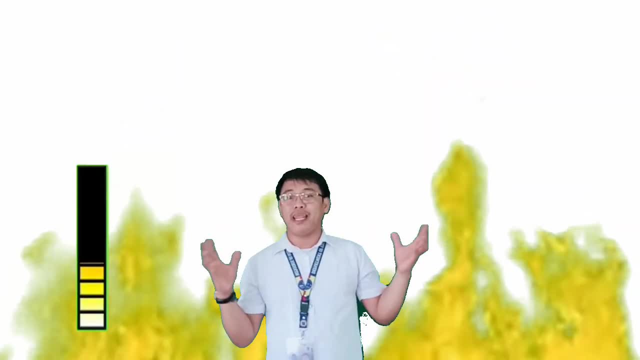 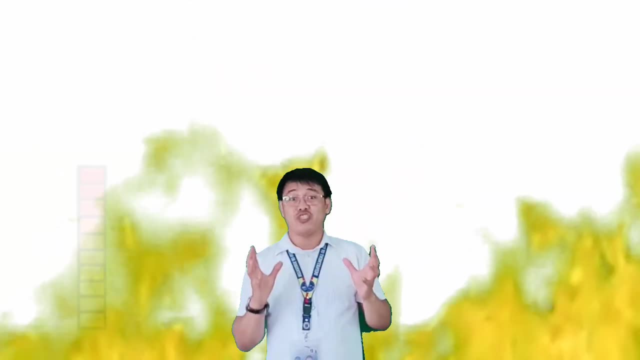 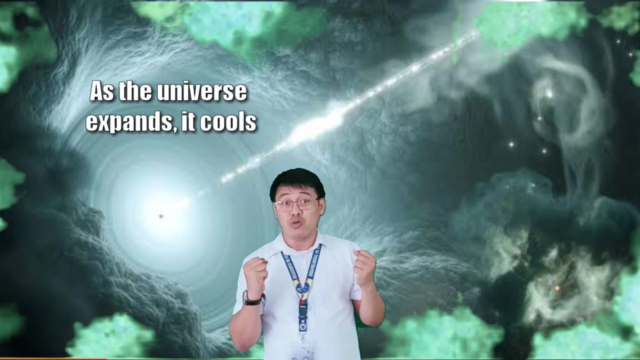 The Big Bang Theory predicts that the early universe was a very hot place, too hot that even the particles of protons and neutrons are destroyed during collision. Since Big Bang is an expansion of space, when the universe expands, it cools One second. after the explosion, the temperature slowly decreases to a point that is enough. 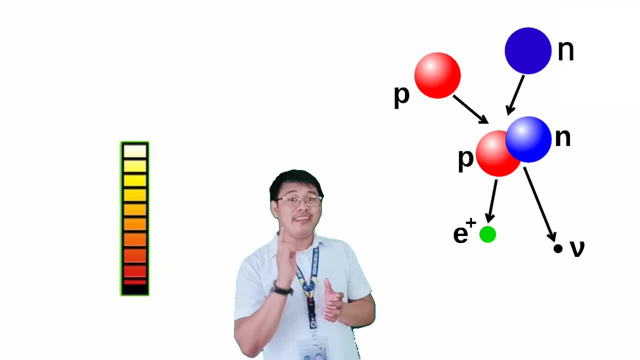 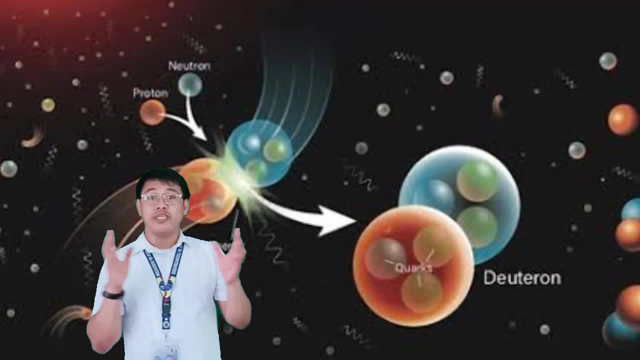 for the protons and neutrons to combine, and that is where the Big Bang Nucleosynthesis begins. As defined earlier, nucleosynthesis occurs when protons and neutrons combine. So when one proton combines with one neutron, deuteron, an isotope of hydrogen is formed. 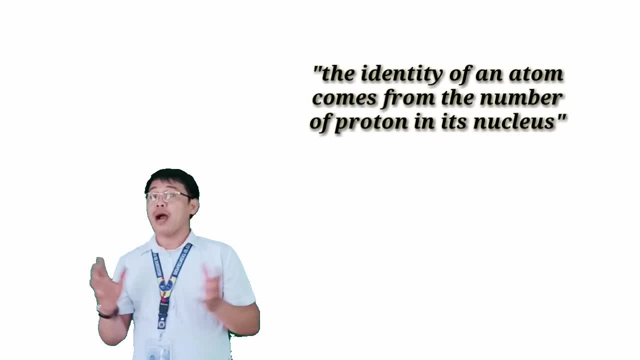 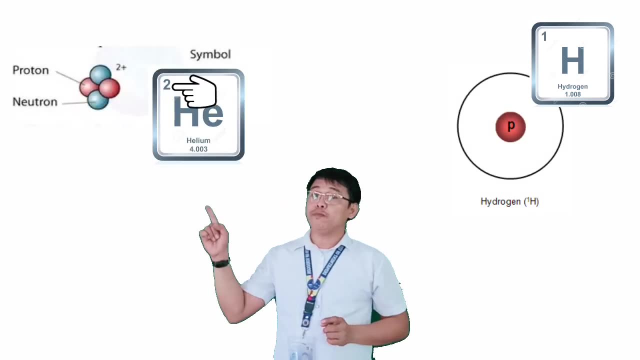 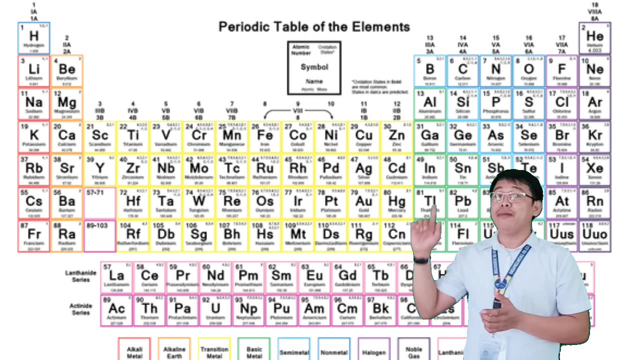 Now remember this: the identity of an atom comes from the number of protons in its nucleus. Hydrogen has one proton, Helium has two protons, Lithium has three, Beryllium has four, and so on. This means that no elements or atoms have the same number of protons. 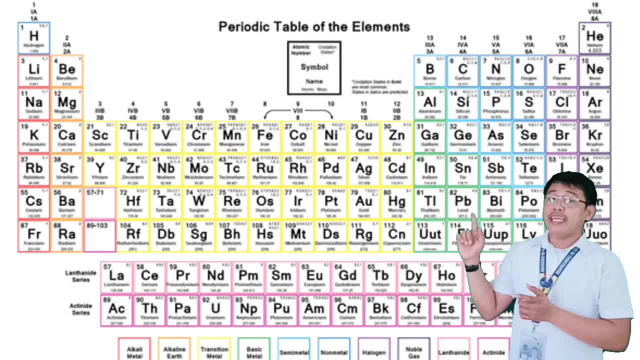 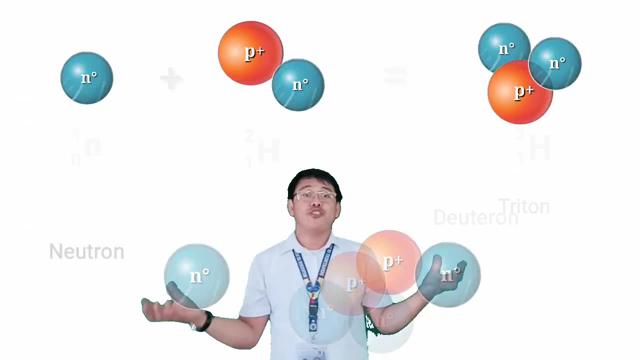 So if you're going to look at the periodic table, the elements are arranged according to increasing number of protons and we call it atomic number. We'll study this further in the next chapters. When deuteron combines with one neutron, triton is formed. 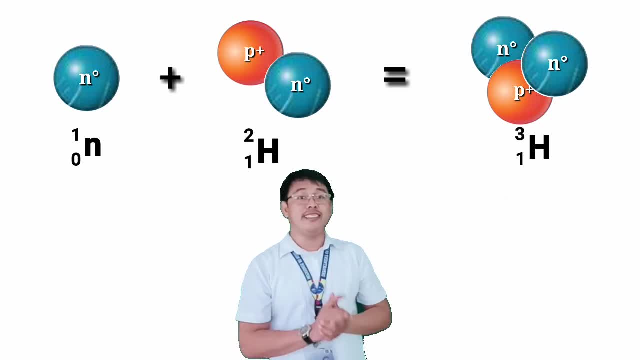 And this is still hydrogen, since deuteron combines with one neutron. And this is still hydrogen, since deuteron combines with one neutron, triton is formed. The reason for this is because it has only one proton, regardless of the number of neutrons in it. 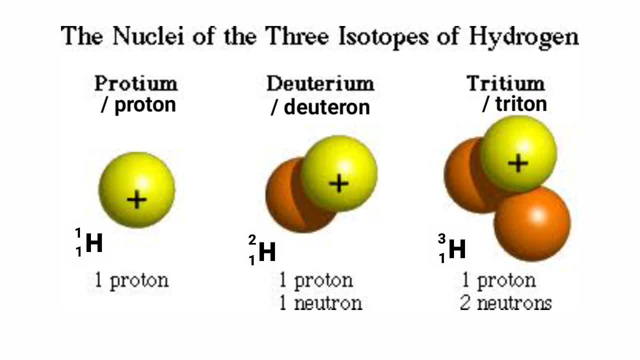 As you can see, hydrogen has three isotopes. We have proton, since one proton can be regarded as the nucleus of a hydrogen atom. Deuteron, with one proton and one neutron. Triton, with one proton and two neutrons in the nucleus. 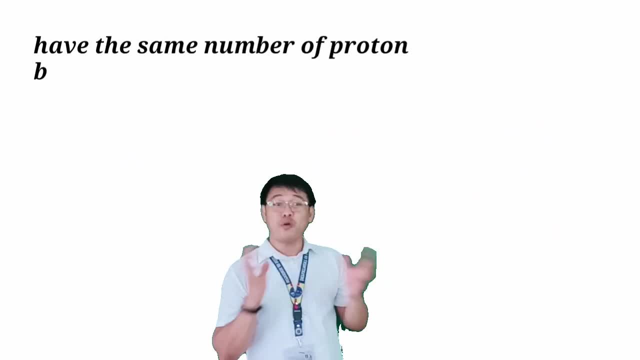 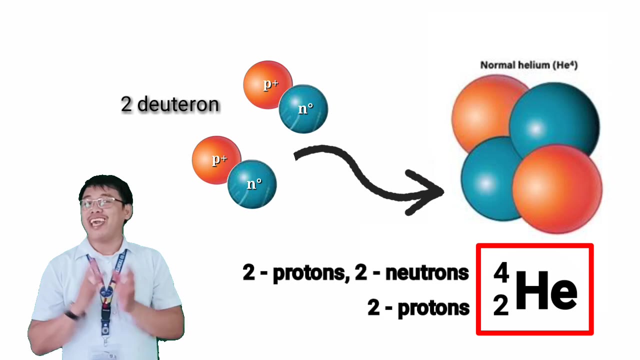 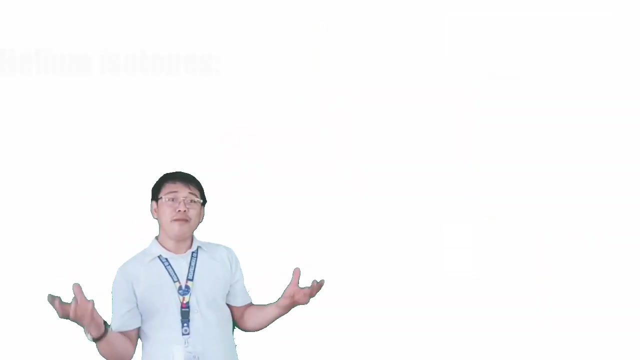 They all have the same number of protons but differ in the number of neutrons. And that is how we define it. an isotope, Two particles of deuteron, can combine to produce helium atom with two protons and two neutrons. When a triton is bombarded with a proton, helium is also formed. So there are many. ways to form helium atom through the collision of hydrogen isotopes. When a helium ion is bombarded with a triton, the nucleons now have three protons and four neutrons. What do you think is the element formed? Correct, Lithium. How about when two helium ions combine? How many protons and neutrons are in?